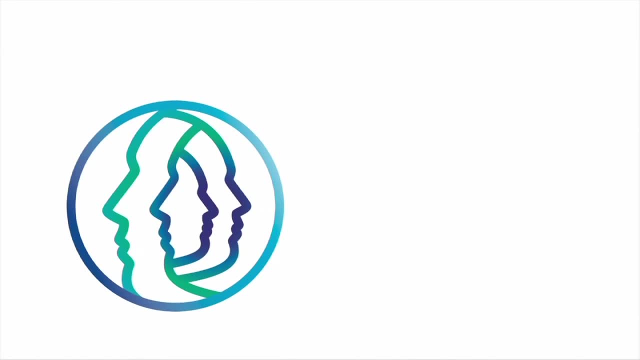 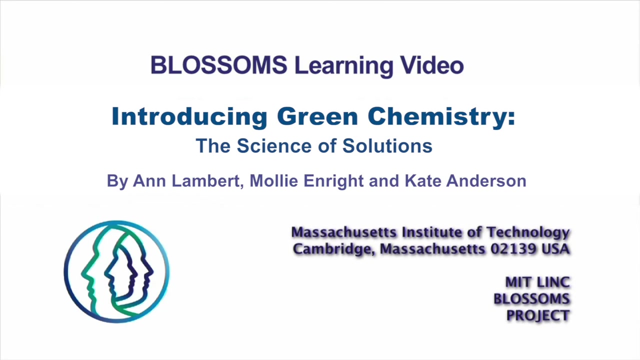 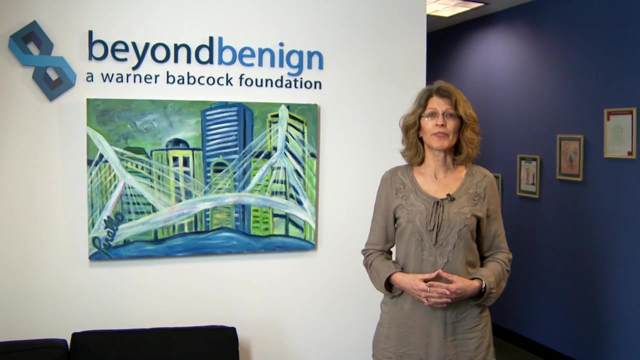 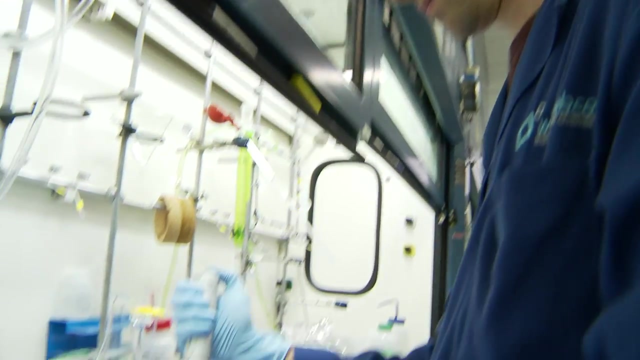 Hello, I'm Ann Lambert, a high school chemistry teacher at King Philip Regional High School in Rentham, Massachusetts, and I'm also a green chemistry lead teacher with Beyond Benign. Today we are on site in the labs of Beyond Benign and the Warner Babcock Institute for 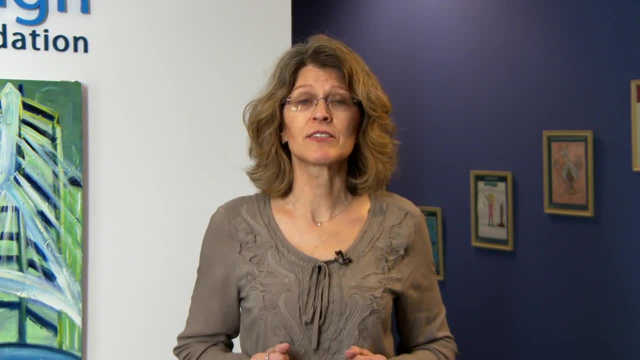 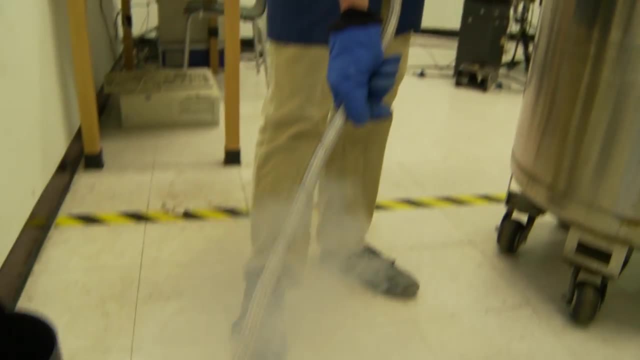 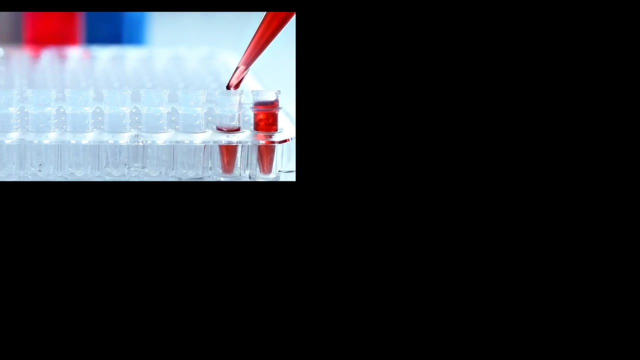 Green Chemistry Beyond Benign is recognized as an international leader in K-12 green chemistry education. Chemistry, as you probably know, is the study of matter and the changes that it can undergo. What kind of things do you think of when you hear the word chemistry? 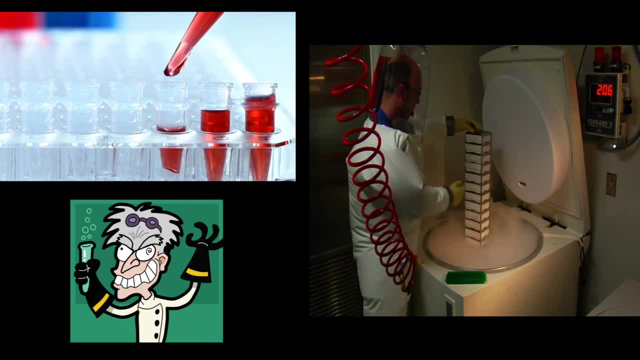 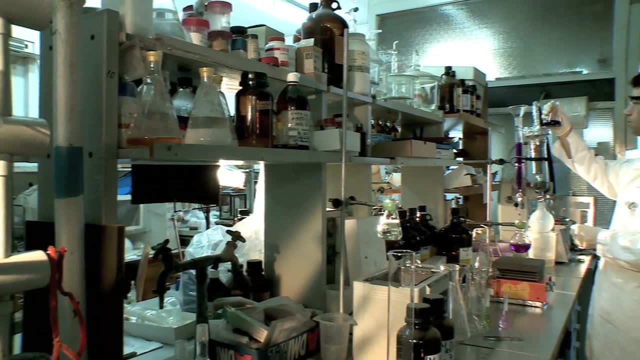 Do you think of some of these types of things? Often, when people think of chemistry, they think of explosions, colored precipitates, reactions giving off toxic gases and other changes that are not really likely very green. So how is a green chemist different from a? 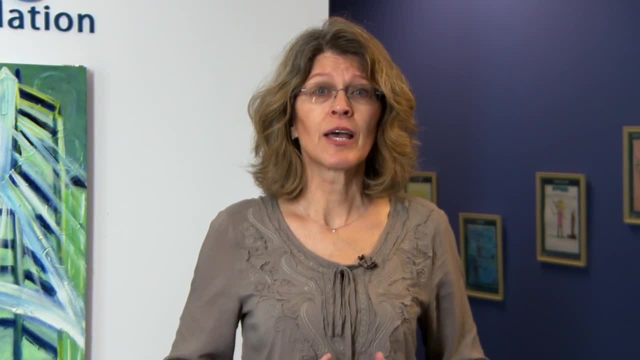 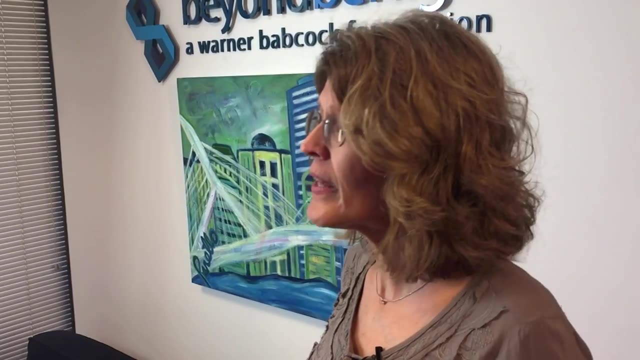 regular chemist. Green chemists still work with reactions and develop new materials, but they make every effort to make sure there are no detrimental effects. Where do you think they look for ideas? One great place is to look to nature. Nature has found a way to. 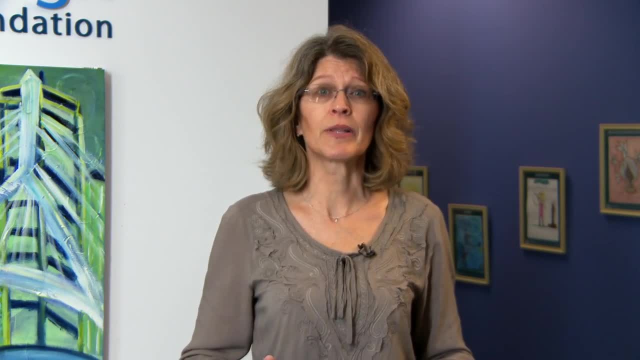 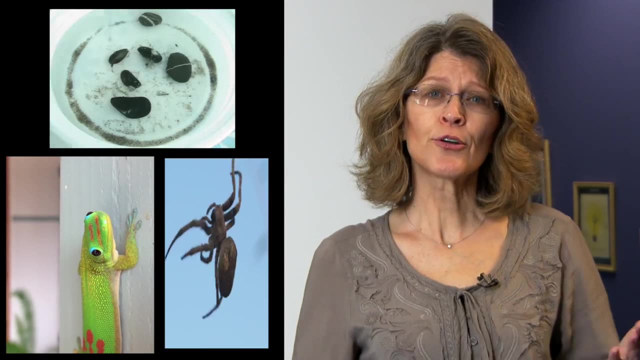 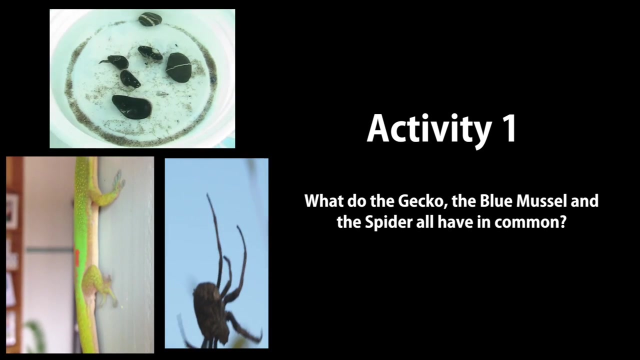 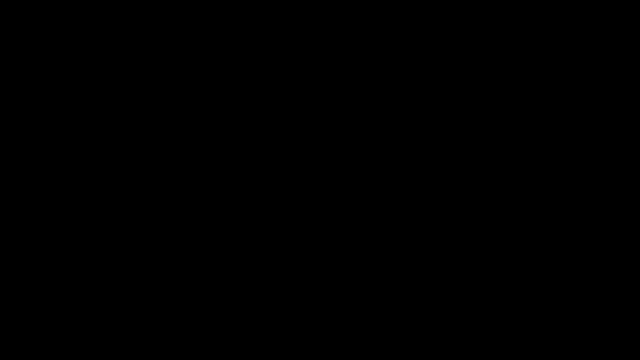 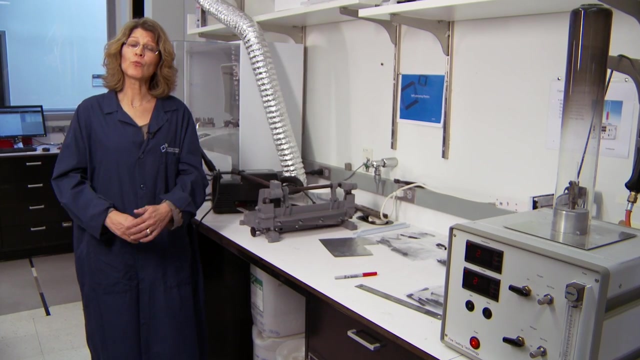 develop chemicals that are non-toxic yet still extremely effective. Let's take a look at some things in nature. What do all these creatures have in common? Turn to your neighbor and discuss what you think. Welcome back. We're now in one of the labs at the Warner Babcock Research Institute for 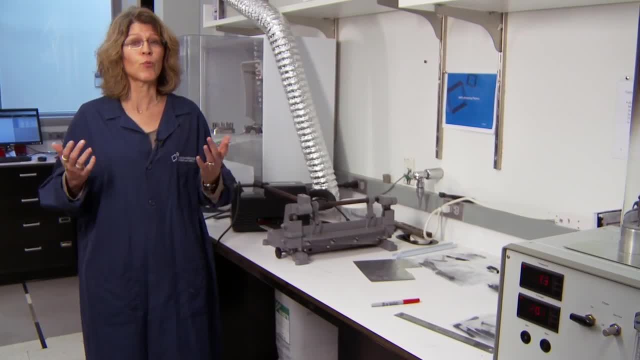 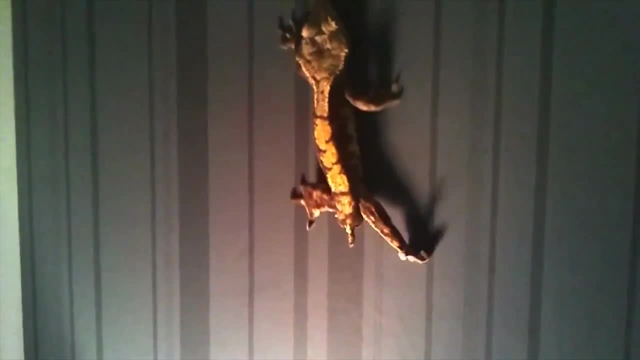 Green Chemistry Did you come up with a variety of answers for what these creatures have in common. One thing I notice about all these things is that they stick to other things. How do they do this? Interestingly, they do not use a mechanical means: The spider web. 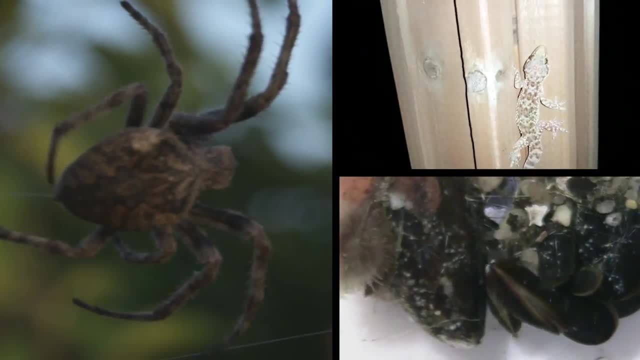 the gecko and the blue mussel all use intermolecular forces to adhere to other substances. This means that they stick to other things using physical means. What is in common? The intermolecular forces or intermolecular forces. These are normally called intermolecular forces in the 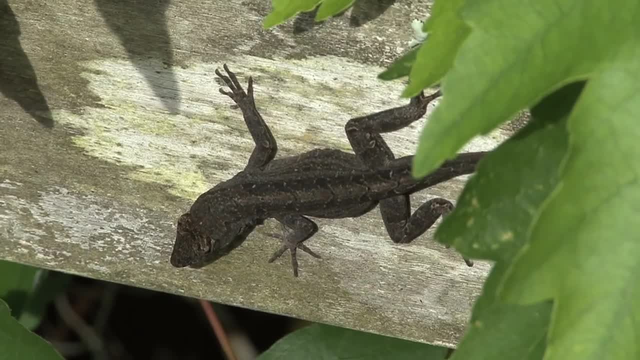 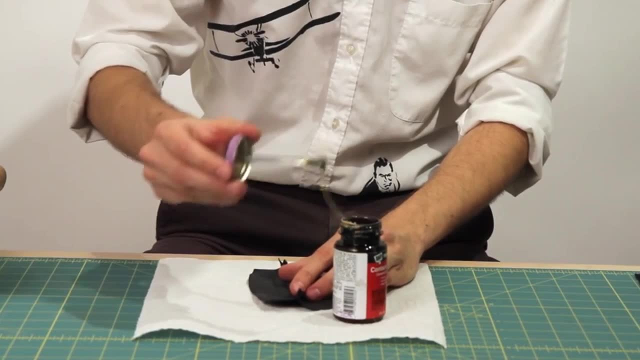 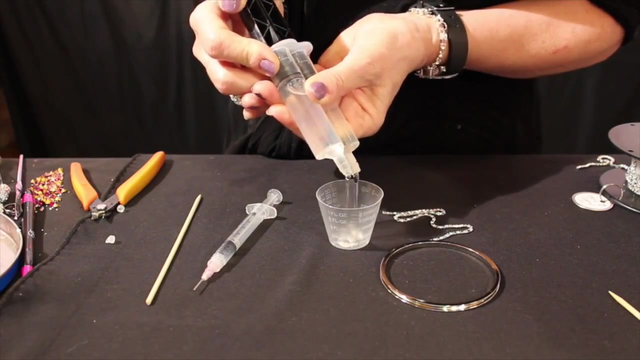 forces between the surfaces rather than hooks or claws kind of like glue, but they do it in a non-hazardous, non-toxic way. Some of the glues that people use are made synthetically using methods that require a lot of energy or involve using hazardous materials. 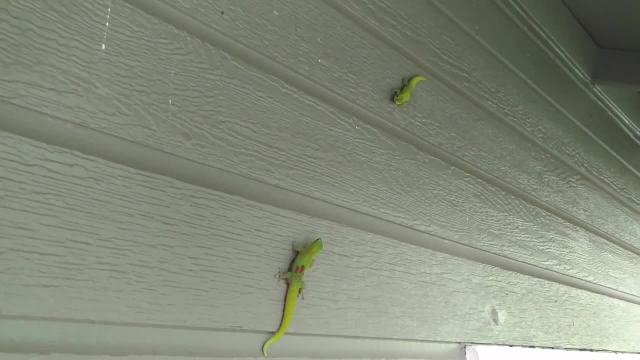 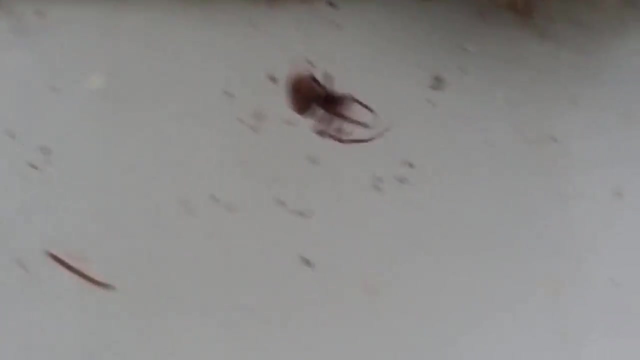 In nature. none of these creatures need extra energy to make their glue, and they are able to achieve a great stickiness without creating any type of hazardous waste. What if we could make a glue that worked like the blue mussels or like the gecko, so that 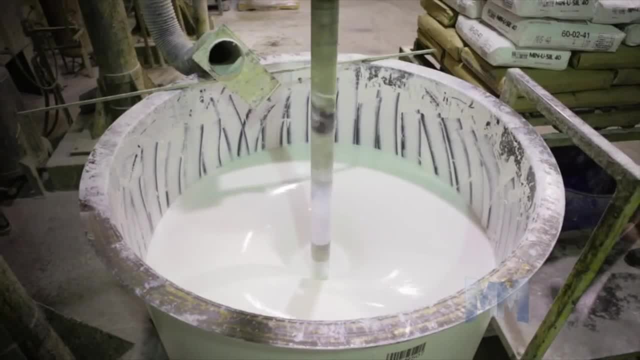 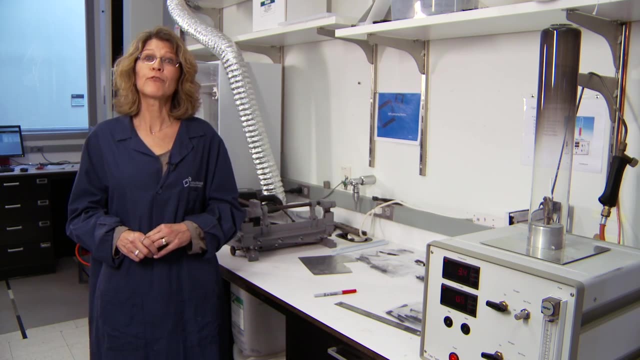 we didn't need to use high energy or harmful starting materials. This is where green chemistry can come in. Now that you've got a little background information, let's brainstorm for a definition of green chemistry. Work with a group or with your partner and come up with an idea of what you think green. 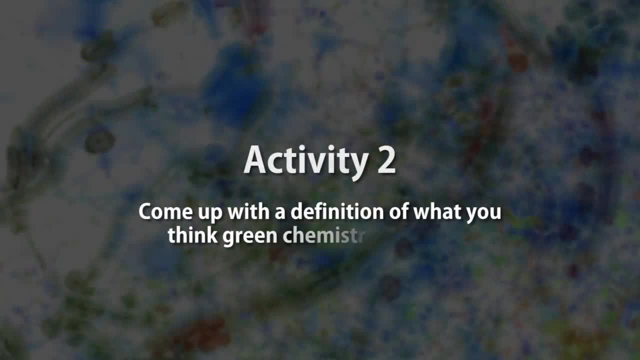 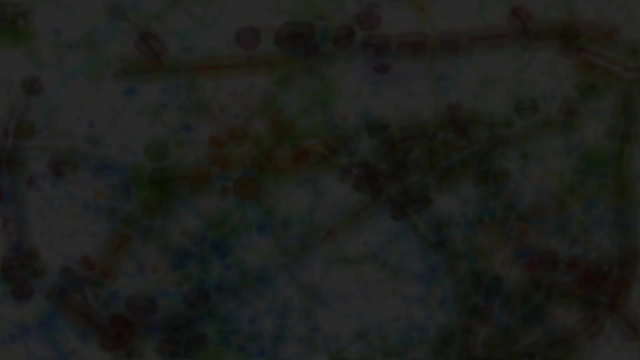 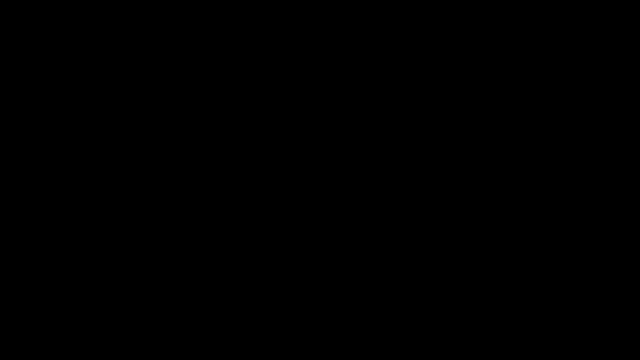 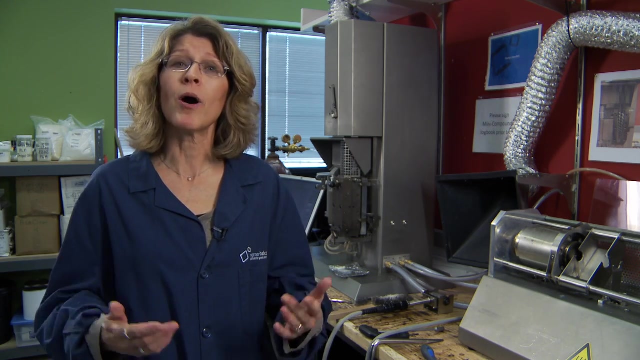 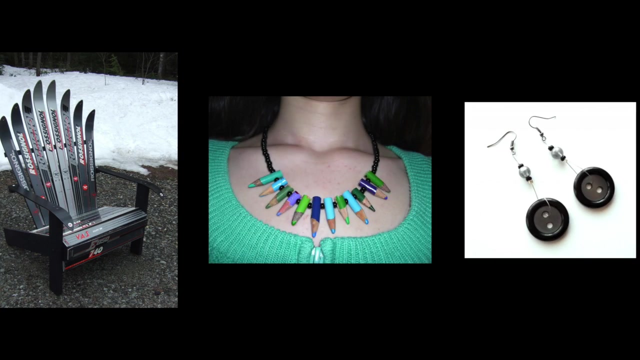 chemistry might be. How was your discussion? I bet you came up with some great ideas about what green chemistry might be. When I think of green, I think of the environment, Things that are made from recycled materials, products that are made from plants. alternative. 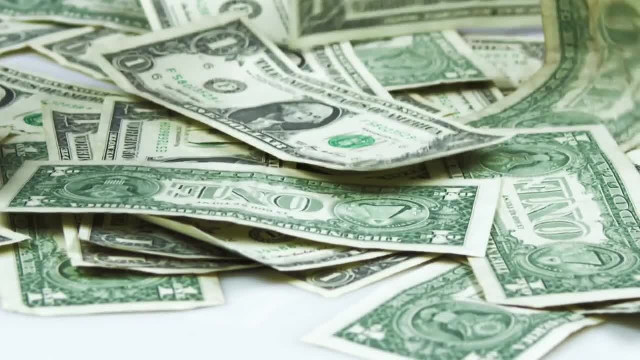 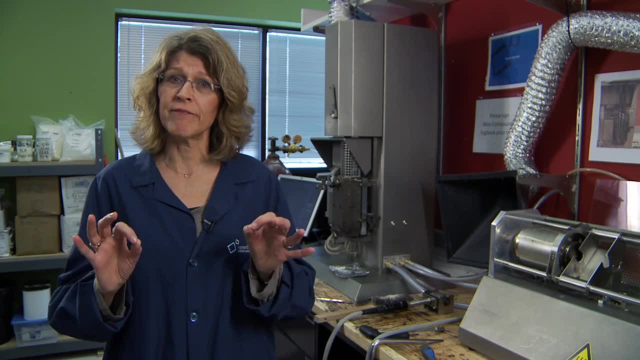 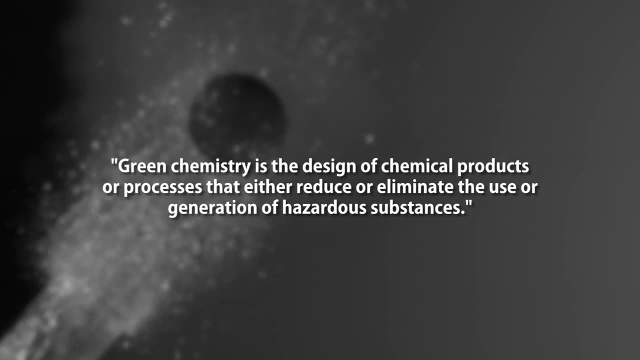 energy. I bet some of you even thought of money when you thought of green. There are lots of ways the word green might be used, but green chemistry is actually very well defined Technically. green chemistry is the design of chemical products or processes that either. 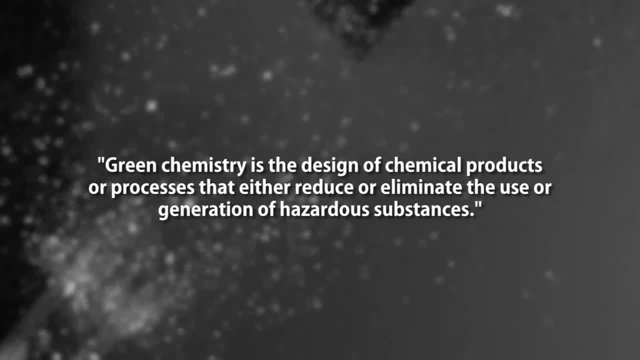 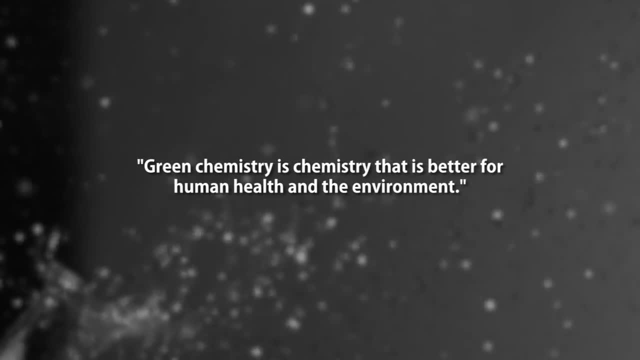 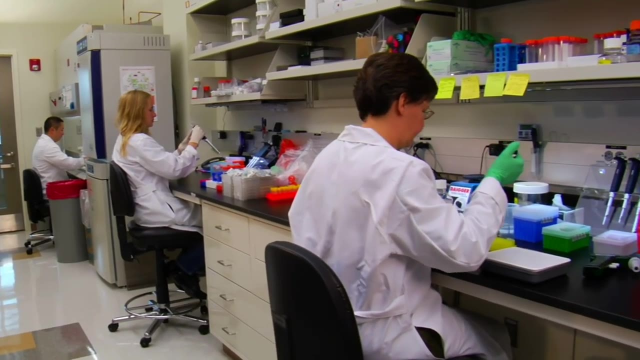 reduce or eliminate the use or generation of hazardous substances. Now that's a pretty lofty definition, but we can summarize it pretty easily: Green chemistry is chemistry that is better for human health and the environment, And oftentimes this type of chemistry can actually save you money, because we can. 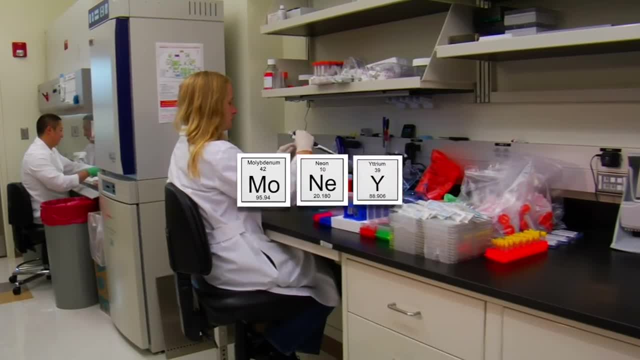 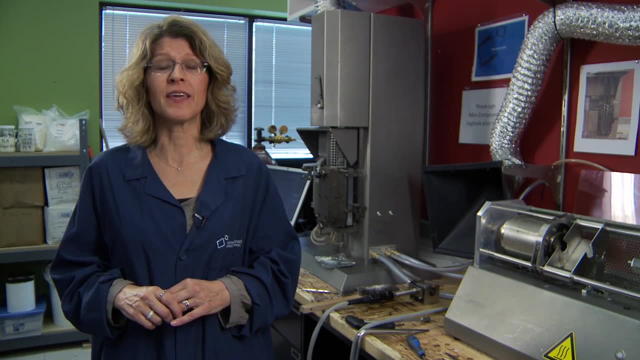 decrease the cost of waste and hazard management. So, those of you that thought about money, you're not wrong. Okay, let's get ready to do a lab activity that will help us to think about green chemistry. You're going to make some homemade glue. 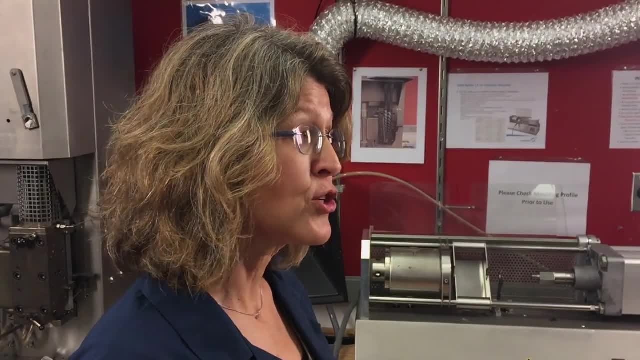 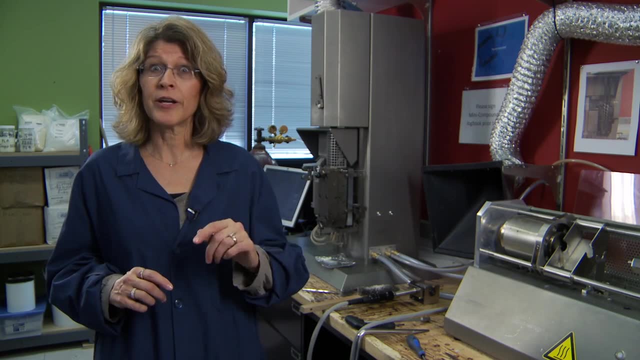 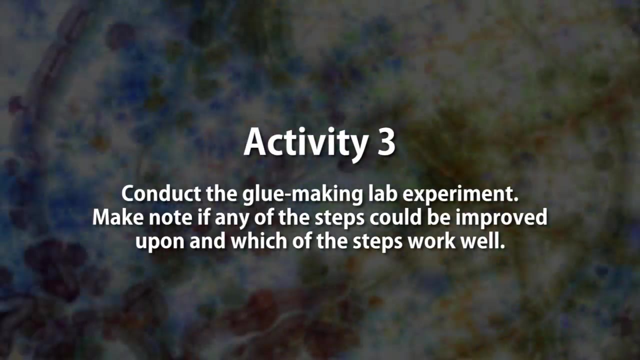 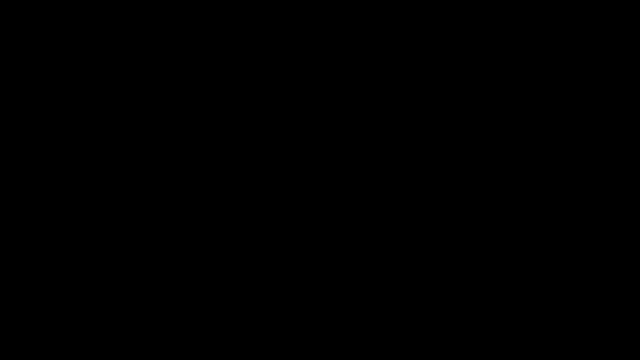 You're going to be given a handout with some lab directions. Make sure you follow them step by step, but, as you're doing it, make note if there are any that could be improved upon. And, while you're at it, make sure you note which steps work well. 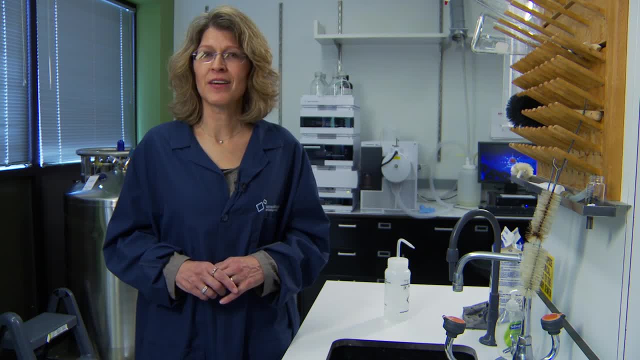 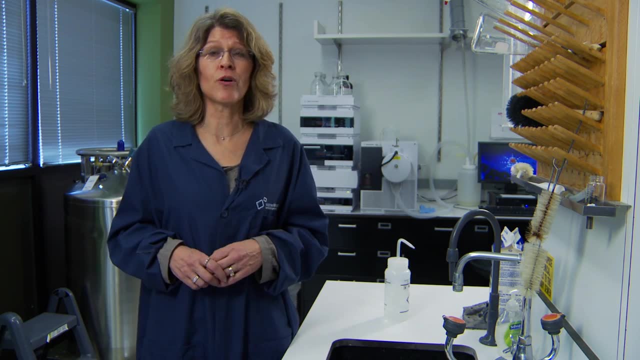 How did your glue come out? What'd you think of some of those steps? Did some of them seem a little Unnecessary, Wasteful, Even silly, Perhaps even dangerous or harmful? If you thought so, I definitely agree with you. 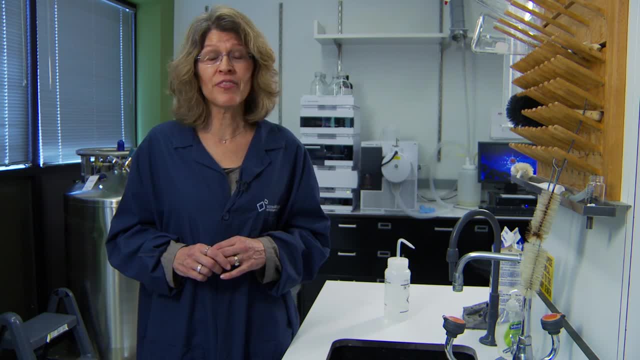 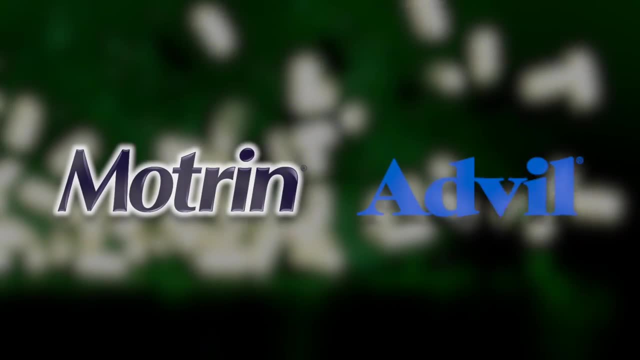 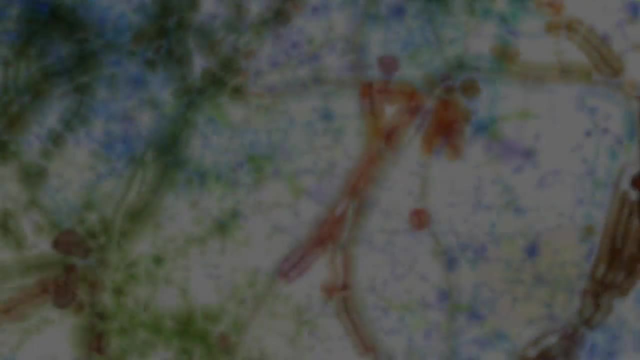 In chemistry, there are some traditional reactions that we could think the same thing about. For example, ibuprofen, the painkiller now known by the names Motrin or Advil, was traditionally produced or synthesized with a reaction that involved a huge number of steps. 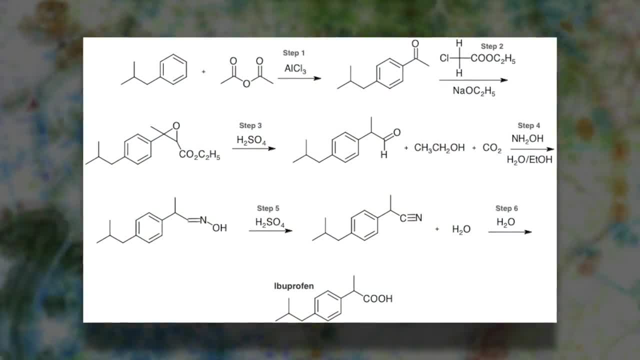 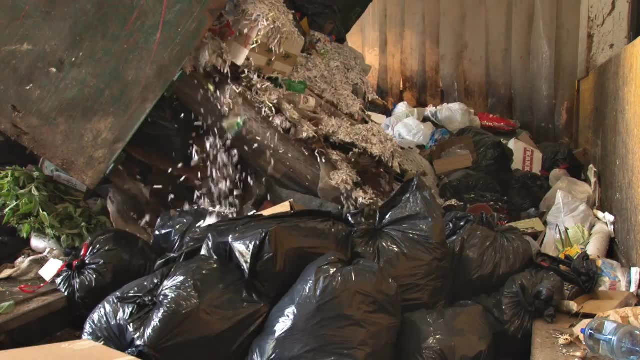 With this process, many of the atoms that start to form are going to be used to make the glue. The glue that started out in the reactants ended up as waste products. With many traditional industrial processes this is the case, and sometimes those unuseful. 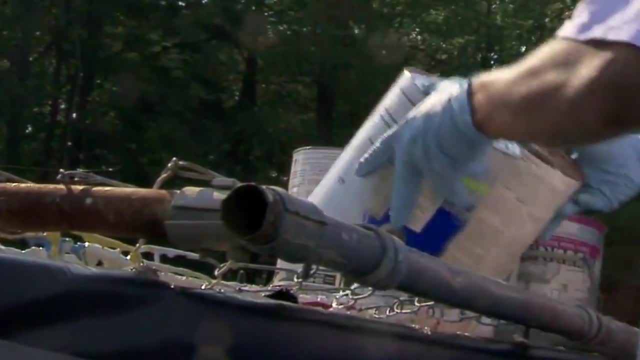 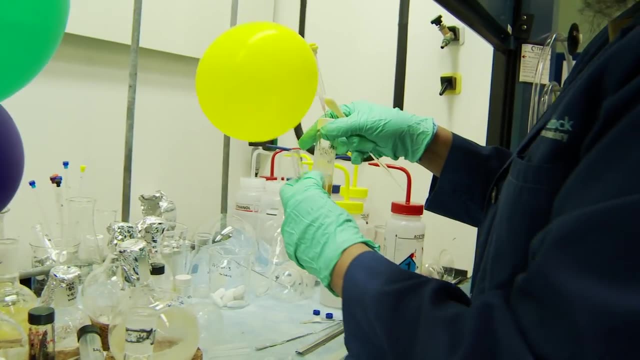 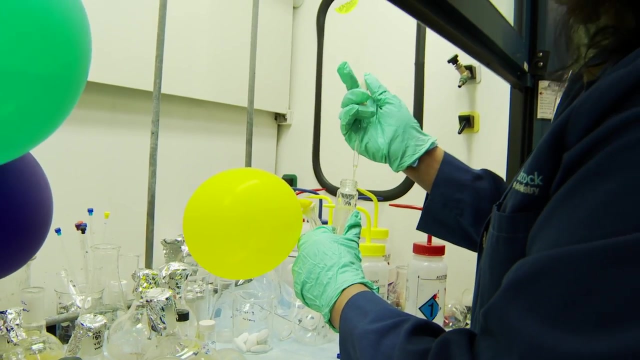 products not only become unnecessary waste, but they are also harmful to the environment or to living systems. As green chemists, it's important not just to think about the properties of your final product, but about the process of making your product as well. 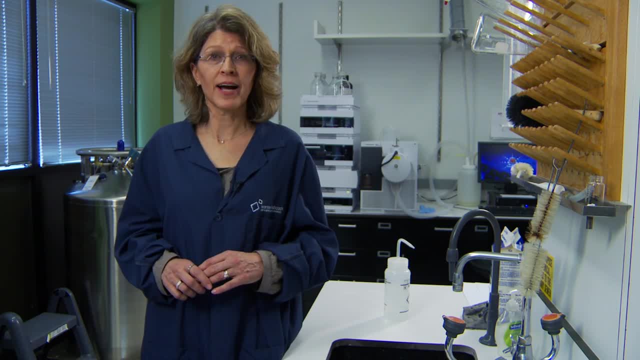 Now it's your turn to be a green chemist. You'll be given a revised lab procedure handout. This is your opportunity to give your boss, the lead scientist, some feedback on that glue recipe. Work with a partner to rewrite each step of the glue recipe. 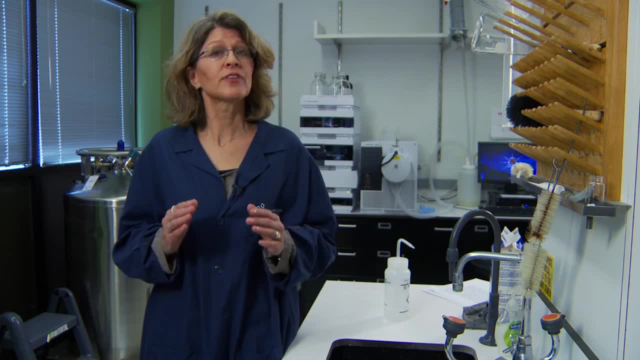 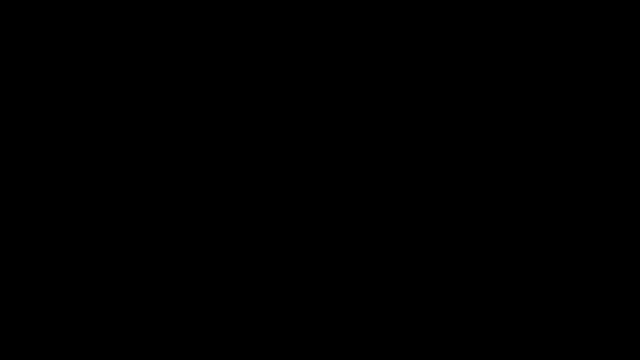 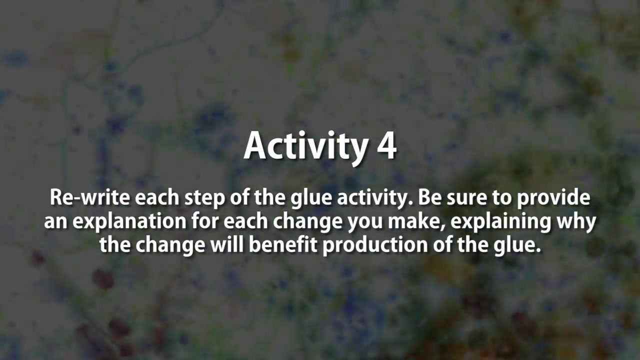 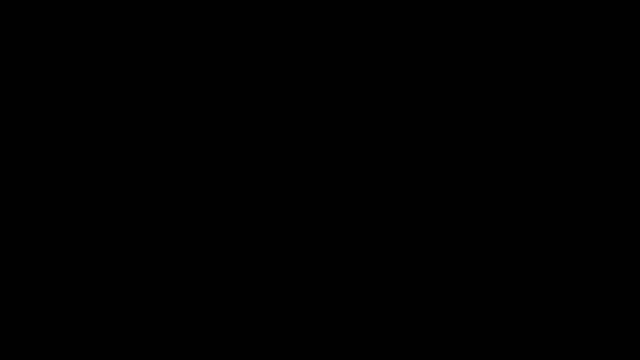 Make sure you provide an explanation for each change you make, as the lead scientist will want to understand how the changes you make will benefit the production of the glue. If you want to have a better look at the results, it's important to get the correct. 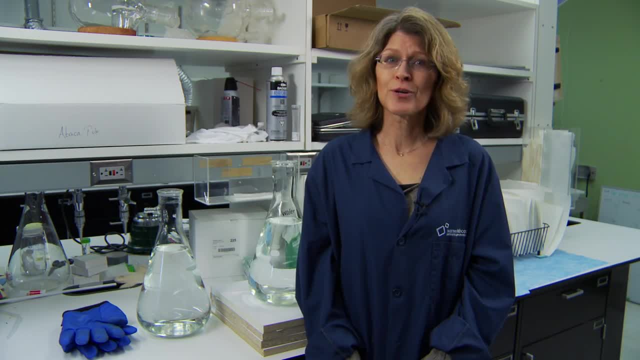 results. How did you do with the revisions to the lab procedure? There were definitely some silly steps involved. Did you all take out the part about singing the alphabet backwards? I'm not sure. if you did, We'll see. You're welcome. 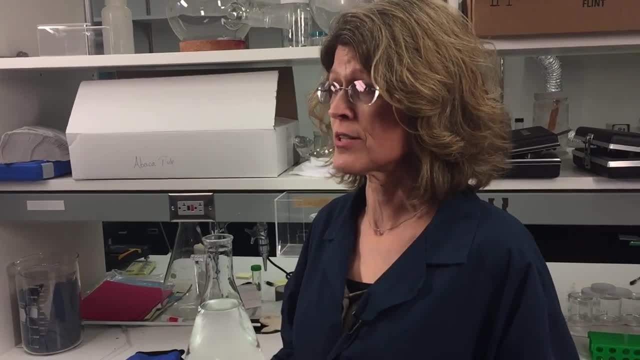 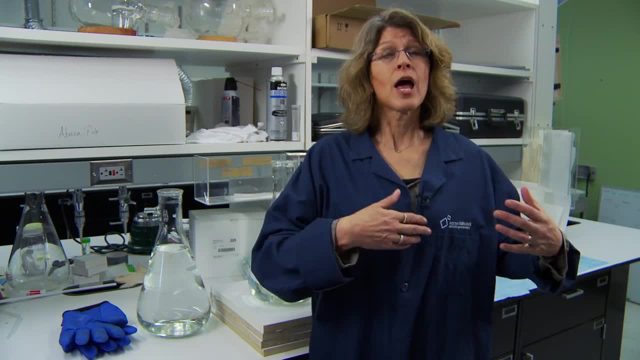 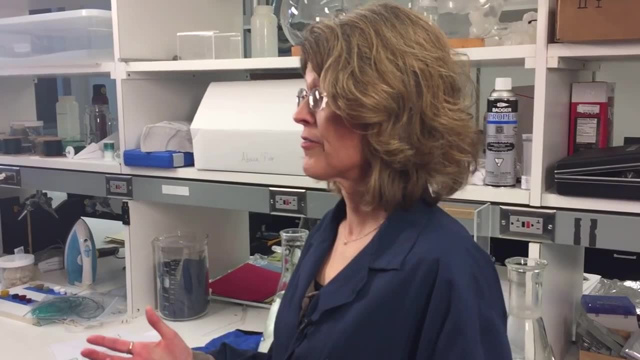 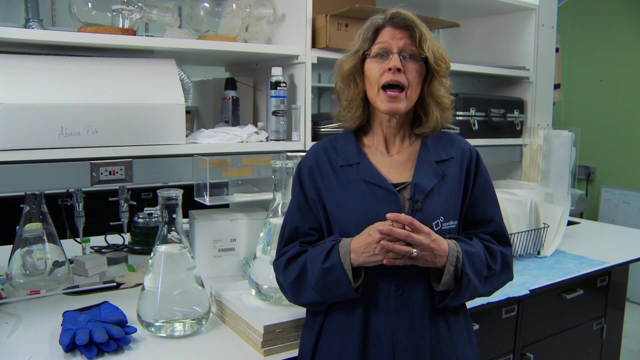 You probably wouldn't give the same justification for not pouring out the excess milk as you would for not reciting the alphabet backwards. There are many parts of our procedure to consider when you're viewing it through the lens of green chemistry. As a class, let's brainstorm how these revisions either minimize the impact on Earth or maximize. 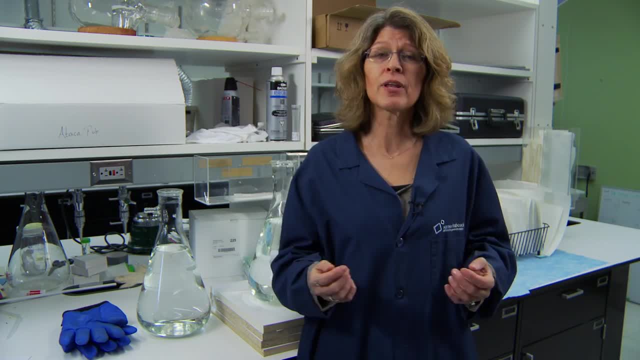 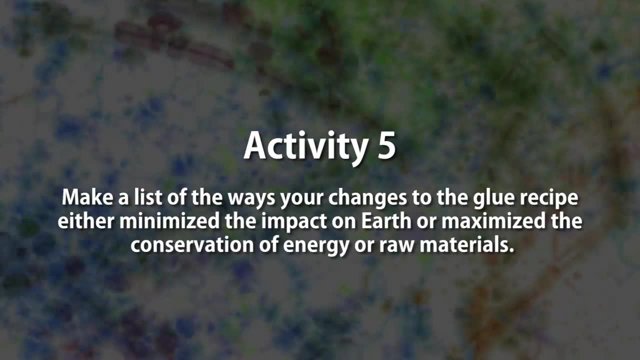 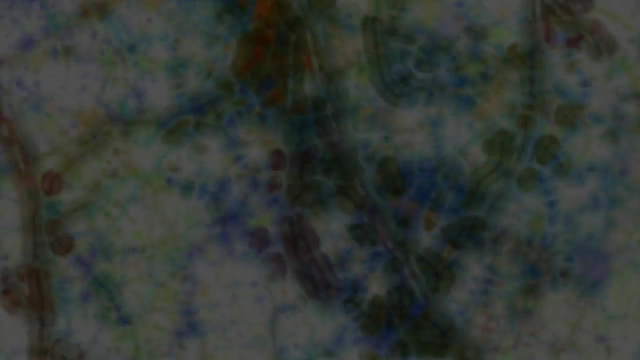 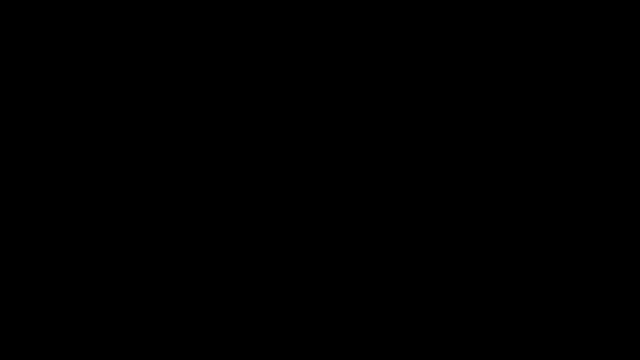 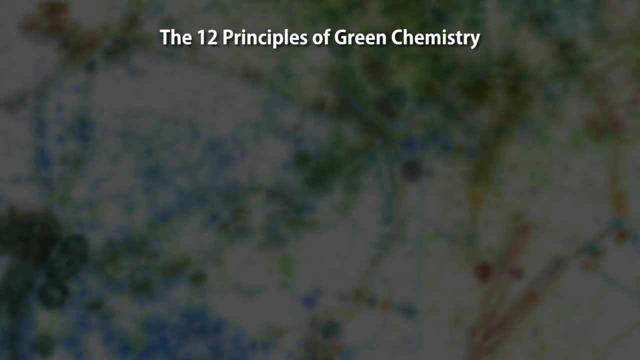 the conservation of energy or raw materials. Perhaps you'd like to write your list on the board. You should now have a copy of the official 12 Principles of Green Chemistry. You didn't know it, but as you were brainstorming a more efficient glue-making process, you 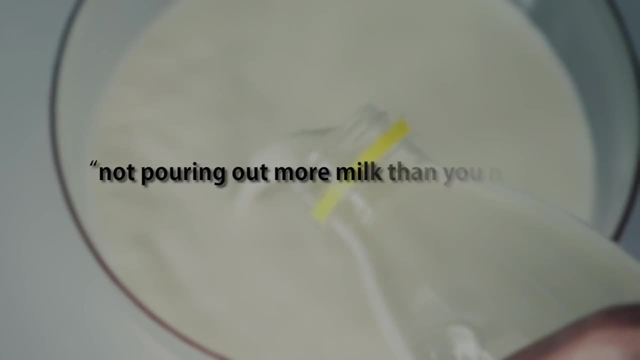 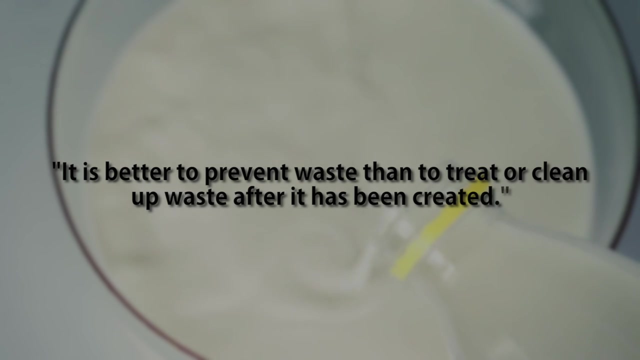 were using the 12 Principles. If you said not pouring out more milk than you need, you were really using the first principle of green chemistry, which says that it's better to prevent waste than to treat or clean up waste after it has been created. 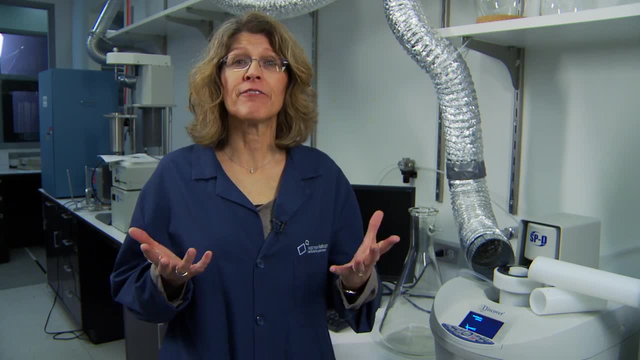 You should now have a copy of the official 12 Principles of Green Chemistry. You should now have a copy of the official 12 Principles of Green Chemistry. If you read the official list of the 12 principles, you might find some of them a little confusing. 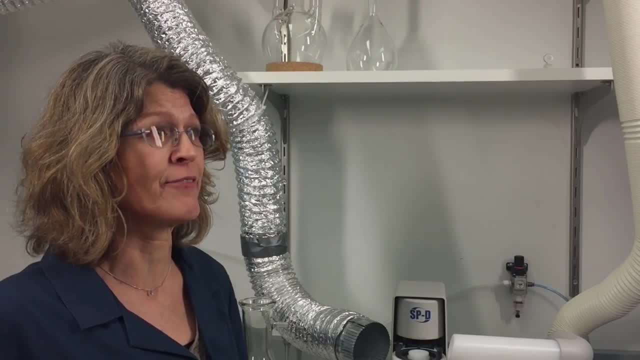 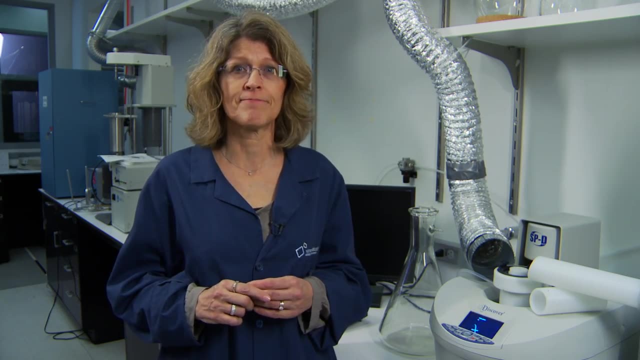 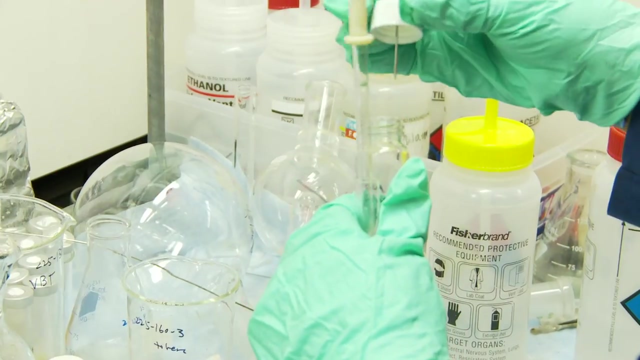 because they're referring to some very complex scientific processes. That's ok, because what you have just done is practice using those principles. Another important aspect of green chemistry is that it has to work as well or better than traditional chemistry. You all have the opportunity to compare your glue with that of a pretty well-made one-on-one. 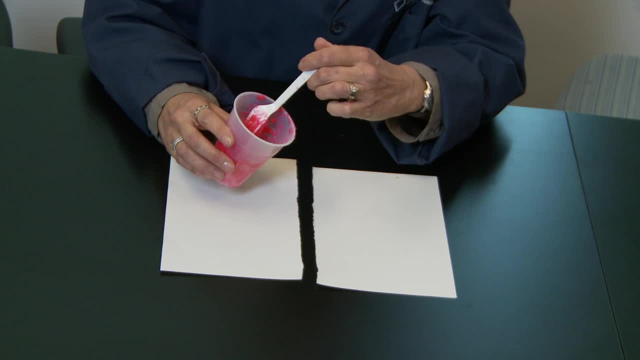 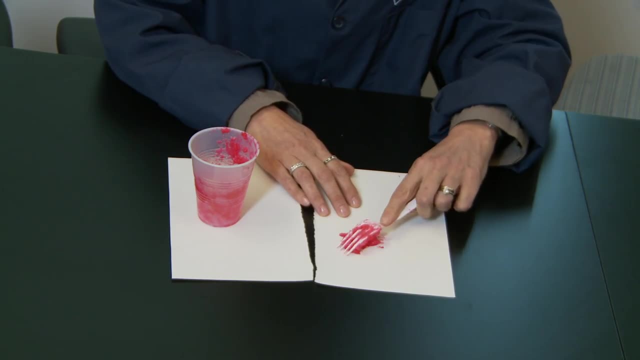 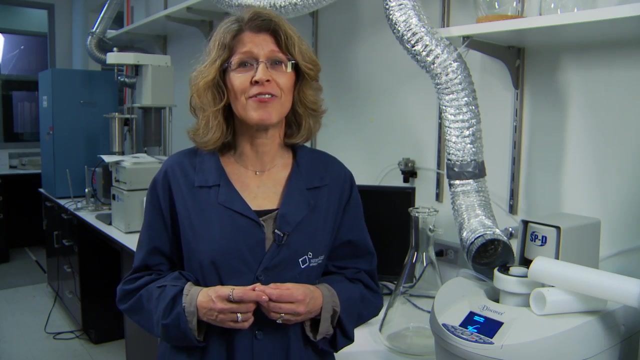 green-chemistry machine commercial glue that you could get from the store By gluing two pieces of paper together with your glue. and gluing two pieces of paper together with store-bought glue, you can compare the quality of your product. I hope that you had some fun. 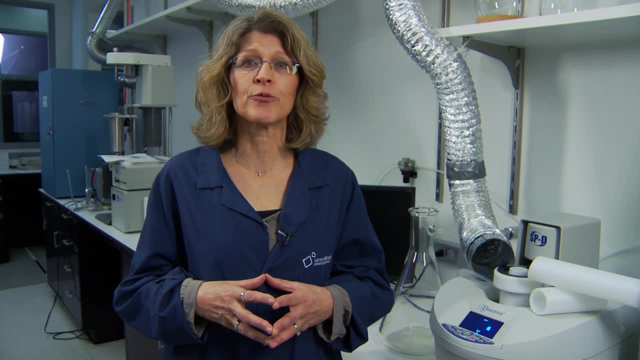 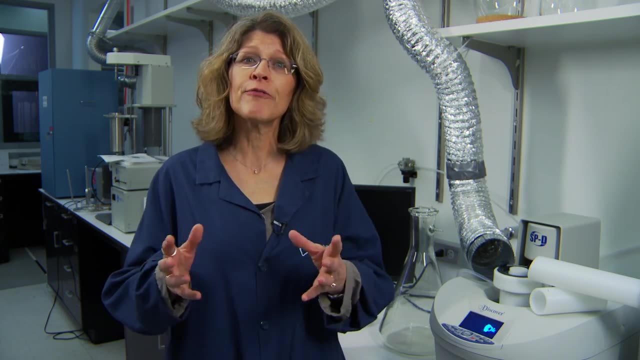 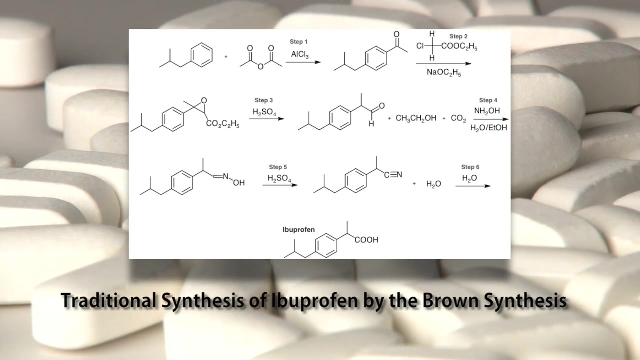 making your homemade glue. Let's summarize what we've learned with this activity. Green chemistry is a process with the goal of doing chemistry that is better for human health and the environment than traditional chemistry processes. If we compare this chart of the traditional steps used to make: 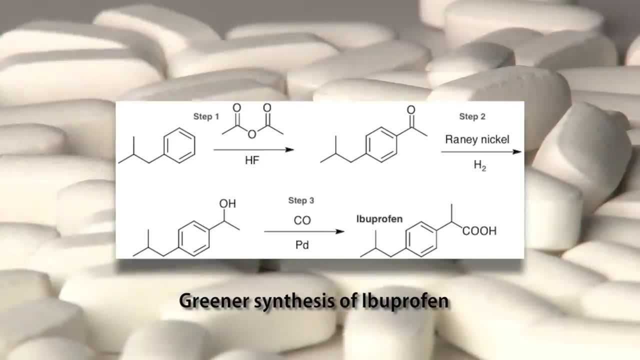 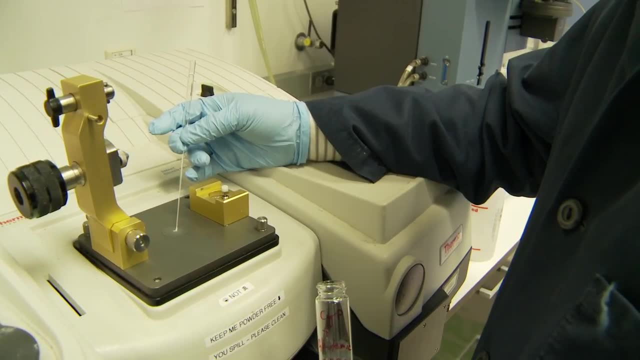 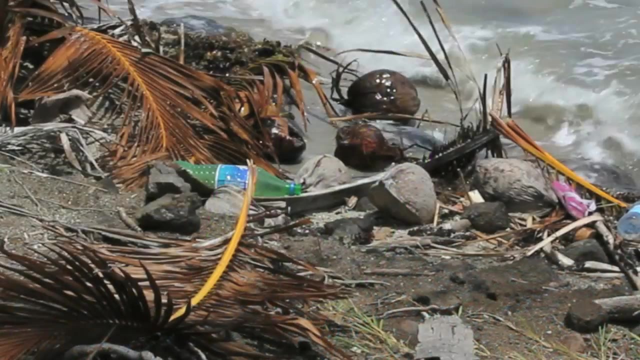 ibuprofen to this revised list of steps that incorporate green chemistry principles, we can see how green chemistry is being used in the real world today to solve many of the challenges facing the environment and human health. Green chemists are using the principles to address issues ranging. 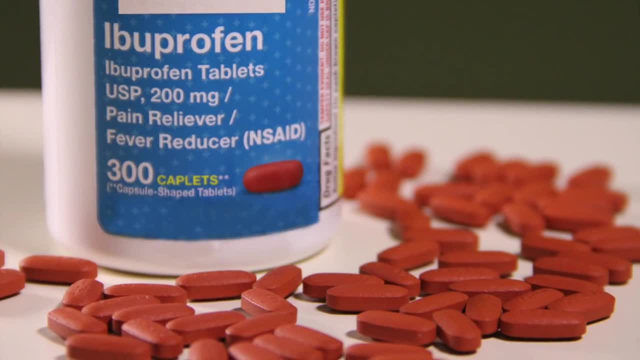 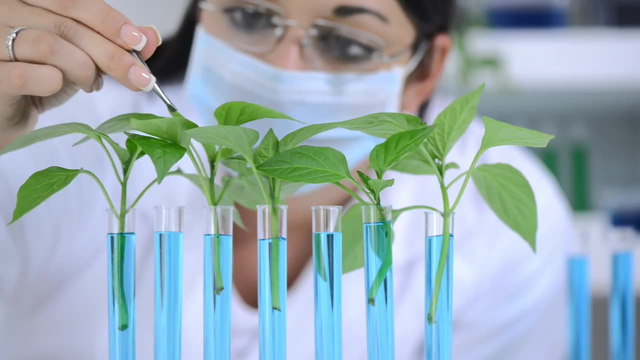 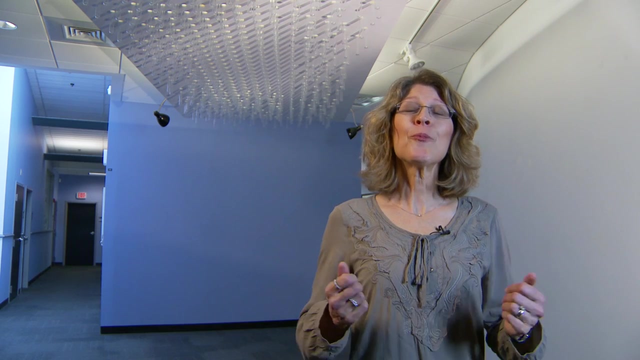 from the problem with plastics in the ocean to pharmaceuticals like ibuprofen. We have a great need for more green chemists who will be able to work to solve many of our problems, as well as create new products that will reduce the amount of waste in our environment. I hope you. 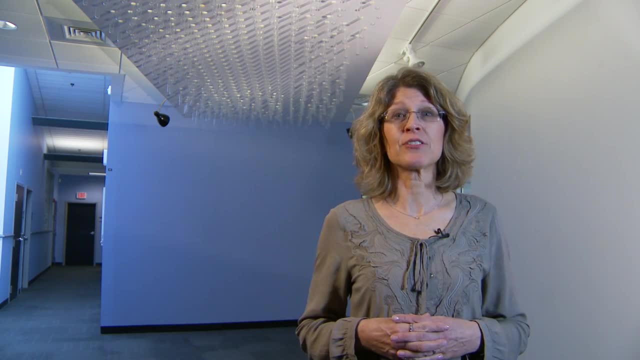 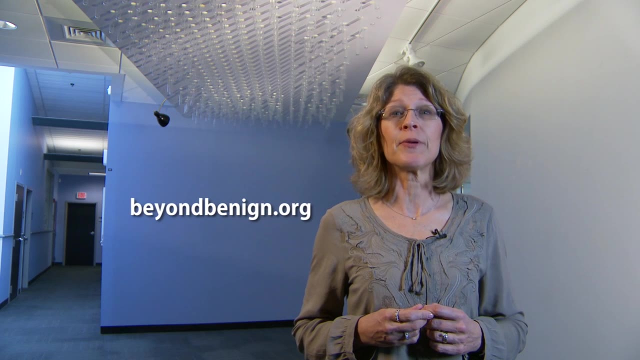 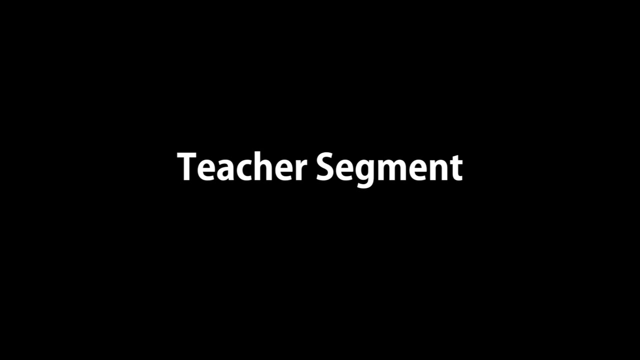 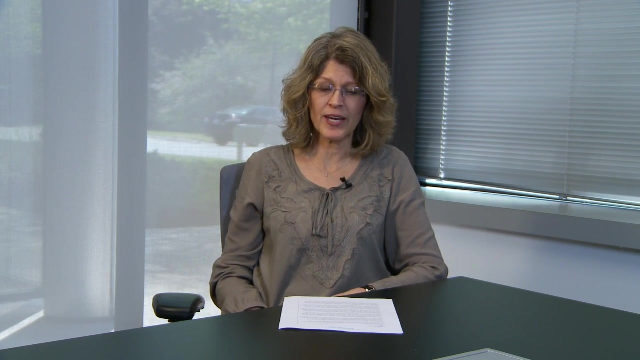 enjoyed making your homemade glue, and this introductory lesson on green chemistry. You can learn more about green chemistry and the opportunities available for a green chemist on the Beyond Benign website. The objectives of this lesson are to introduce students to the ideas of toxicity and environmental impact as it relates to the properties of matter and 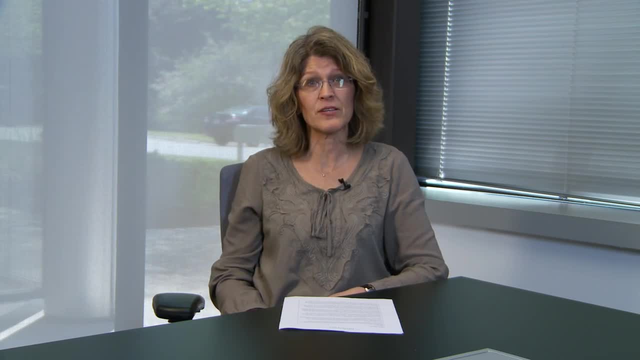 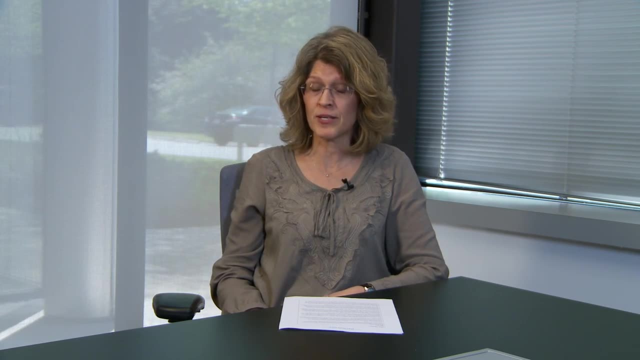 to give students an introductory understanding of the basics of the 12 principles of green chemistry. We want them to be able to use match and measurement to understand the concept of a recipe as it's applied to a chemical process And to give the students a chance to think critically about how the process 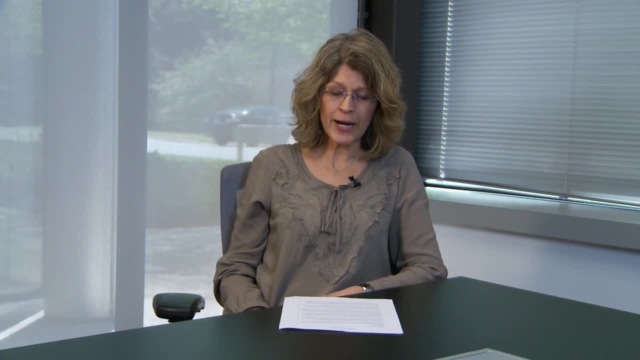 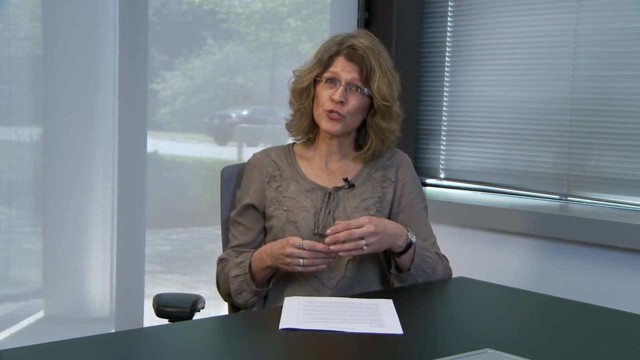 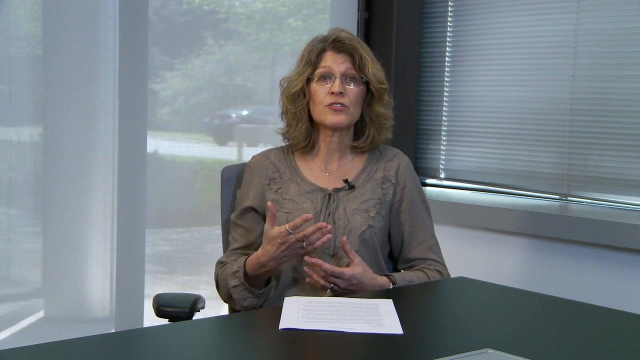 might be improved. The estimated time required for this activity is 60 minutes. You could certainly divide it up into two lessons, whatever fits your schedule better. For example, you could complete the lesson through the glue making activity and then have the students glue papers together overnight, then come back. 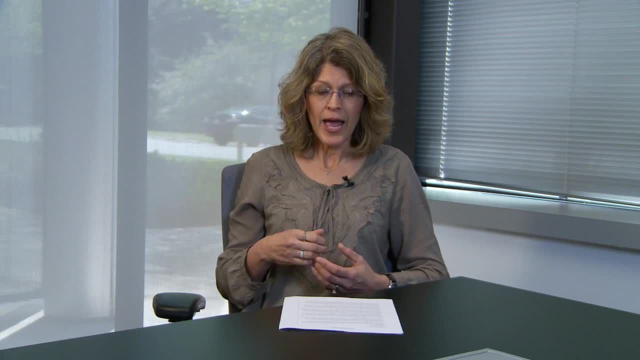 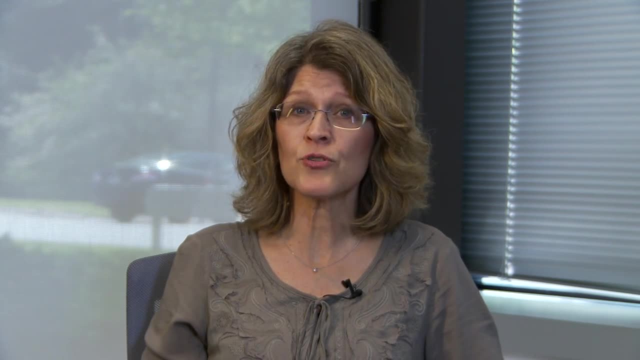 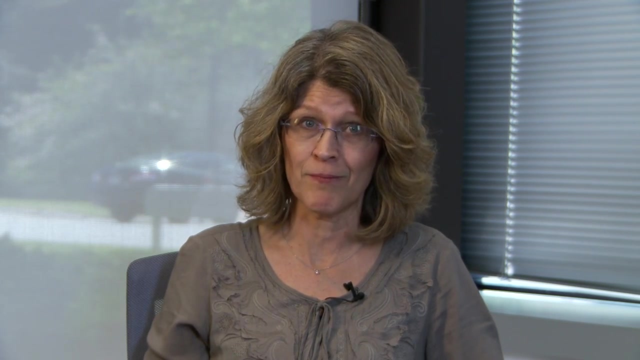 the next day, test the efficacy of the glue and then move on to the brainstorming activities of segment four. The core of this lesson is to have students work through a poorly designed procedure and then have them rewrite the procedure in a way that makes more sense to them. By doing this, the students will naturally make the 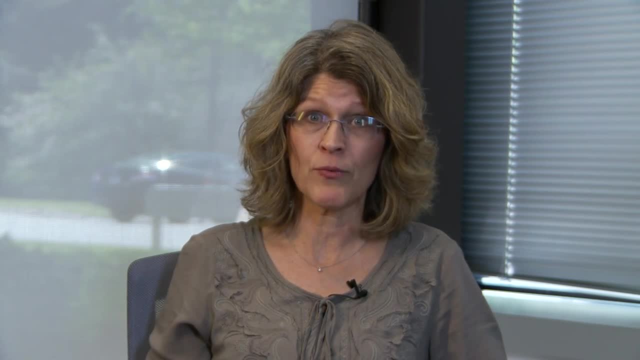 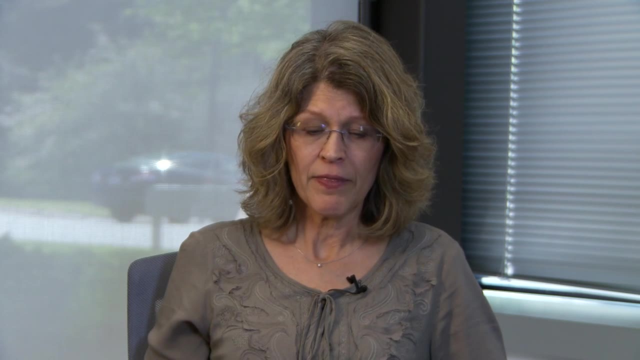 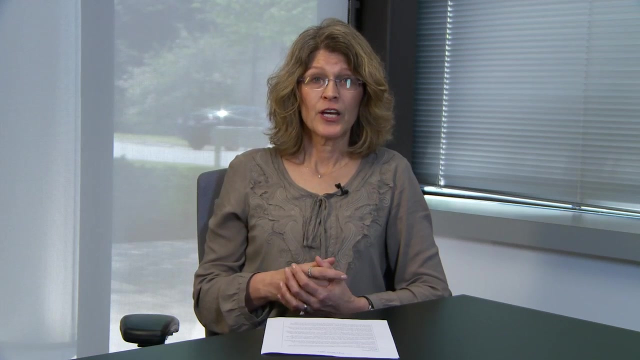 process more natural and less wasteful than that. what was given to them? By asking the students to explain why they made the changes that they made, they are going to be able to fill out a simplified version of the twelve principles of green chemistry together. During activity three, the students could 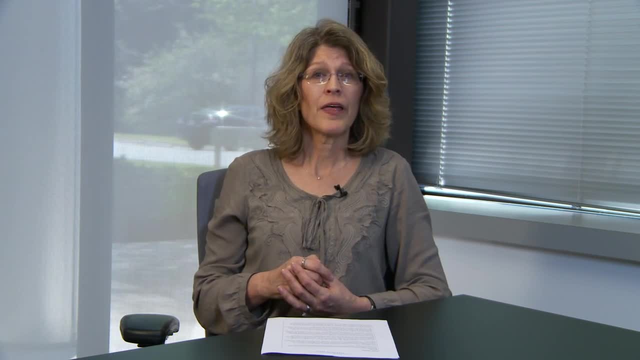 work in pairs or, if more convenient, in groups of four. They may protest some of the steps, which is that they're silly and pointless, but do your best to try to get them through the entire procedure. However, you obviously know your class. 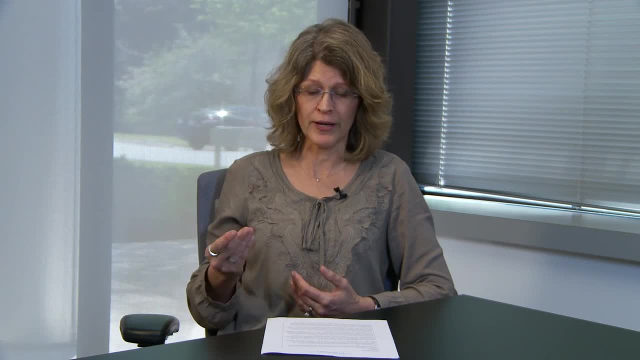 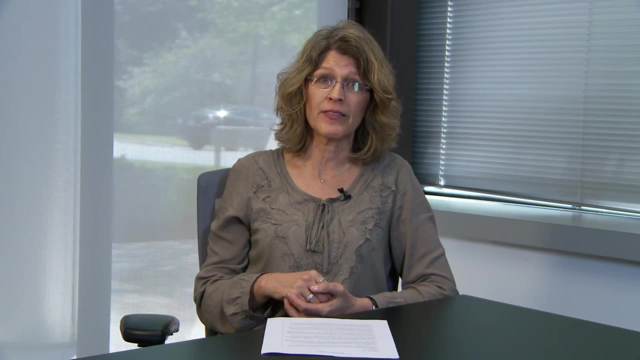 best. so if you think it's better to stop the activity, go ahead and do so, and then you can move them on to the next step. They're going to segment four, which will be activity four, where they're going to rewrite the 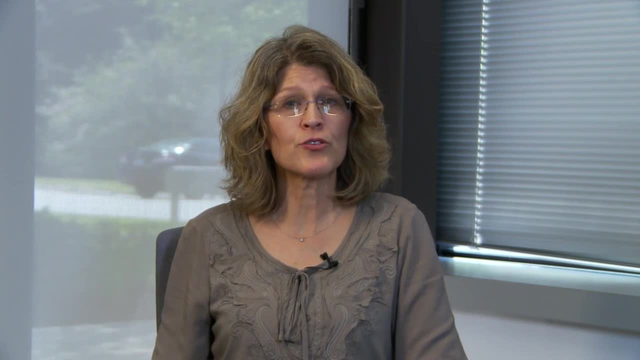 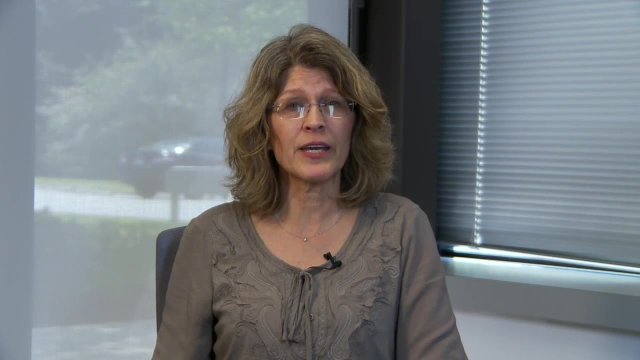 procedure. During activity four students are going to work to rewrite the process. You could have them work individually or in pairs so that they can really think critically about the revisions to the process. Afterwards come back as a class and they can work together to brainstorm, and you want to make sure that they 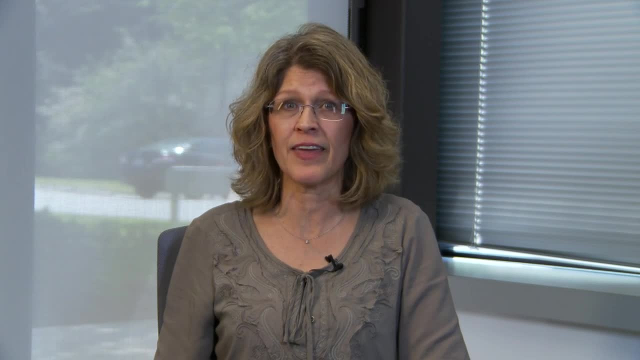 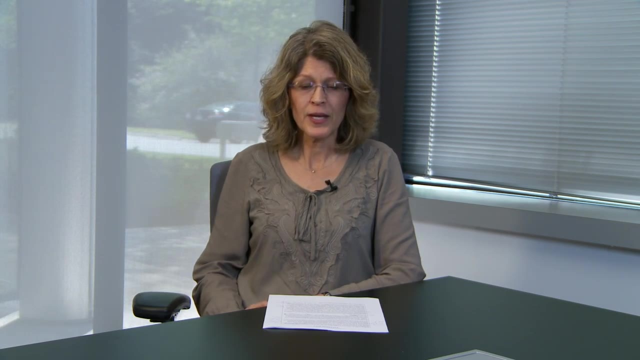 identify the reasons behind the changes that they have made. Activity five will be where you really begin to draw out the take-home message. Together, let the students brainstorm this list of ways that their new versions either minimize the impact on Earth or maximize conservation of materials, or 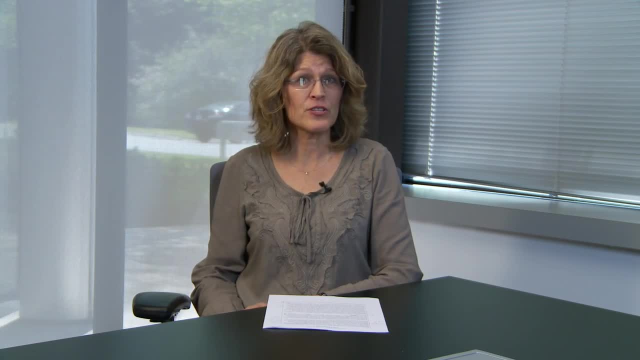 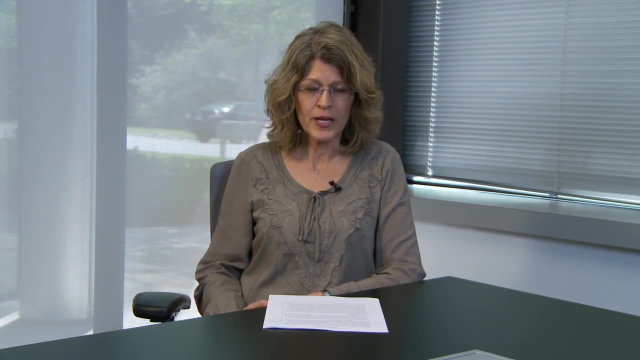 energy. You might want to have them write their list on the board. This is the list from which you're going to draw out the twelve principles of green chemistry. Some of the principles are a bit more complex than the other ones, but they're all very useful. You can use them to create your own. 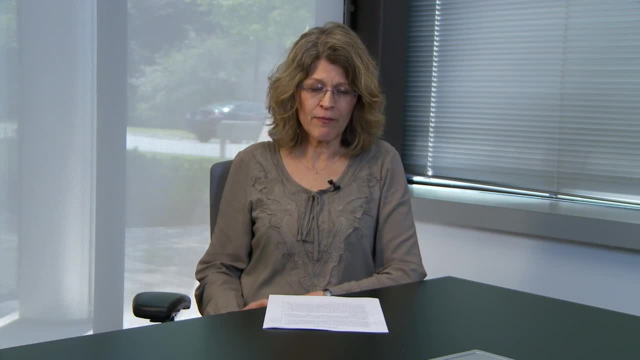 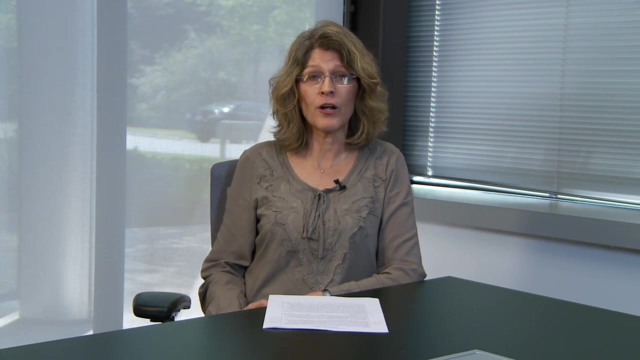 principles. Activity six is a little bit difficult for the students. Perhaps something like principle number eight, reducing derivatives. since they do involve really complex chemical processes, You might need to prompt the students more when you get to those principles, or alternatively, you might decide to just skip some of. 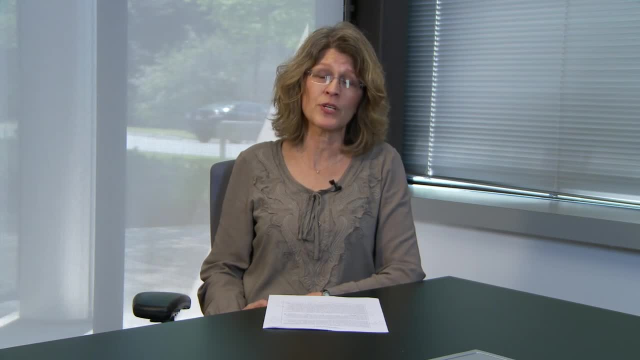 those focus on the principles that your students will be able to understand and relate to, and then you could just give them the more complex principles when you give them the information. In segment six, I'll introduce the twelve principles and showcase how the students have. 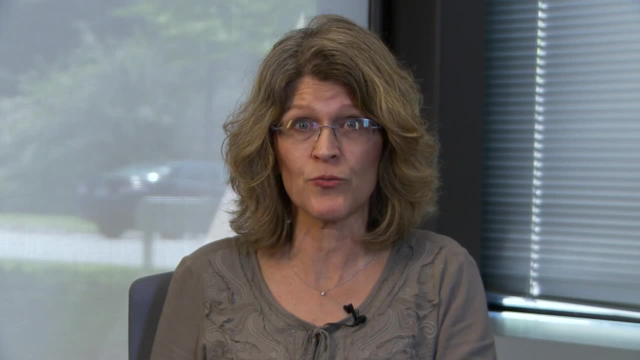 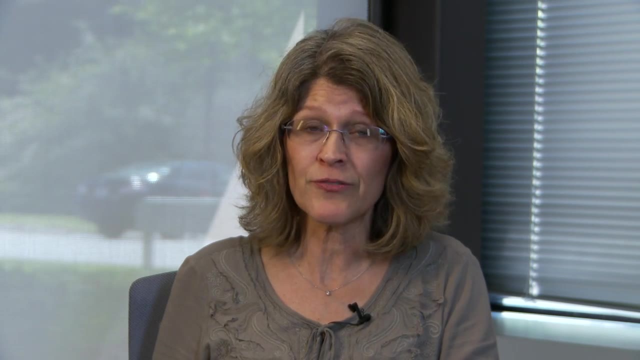 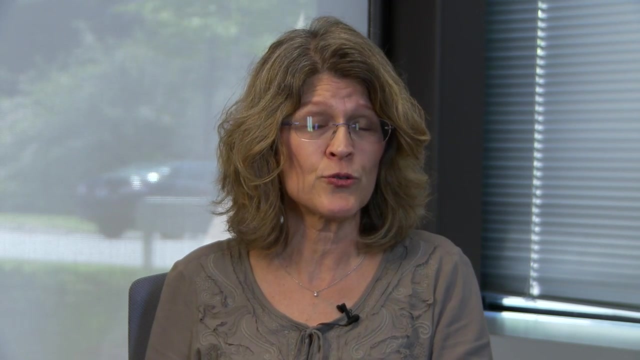 likely already drawn these out through the process that they just went through. The principles were written for complex scientific processes, so they can be difficult for the students to understand and for you to explain. Because of this, it's going to be helpful for you. 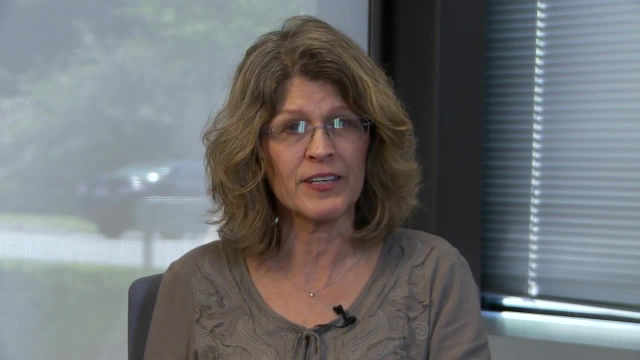 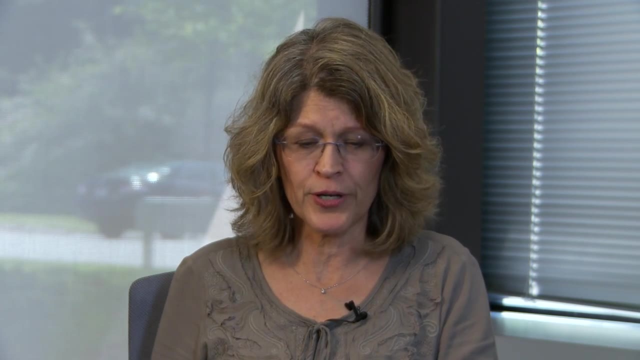 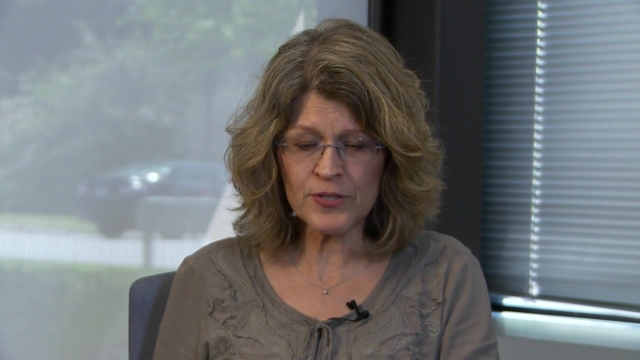 to have read the supplemental information provided in the principles so that you can get the information provided in the teacher background prior to doing the lessons. This will help to break down the twelve principles for you and give you some hints on how you can more easily explain the steps, Though these principles can be complex. the process, 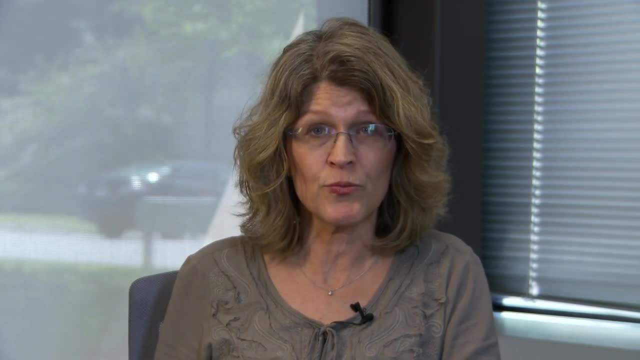 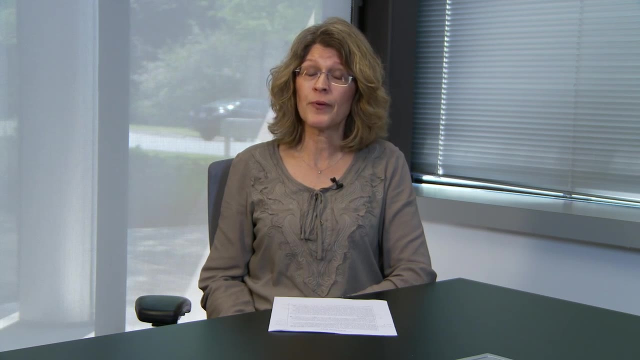 of applying them is going to be exactly what your students will be doing with the glue making procedure. This lesson, as well as all the lessons available on the Beyond Benign website, are available in our website at wwwbeyondbenigncom. For more information, visit wwwbeyondbenigncom. 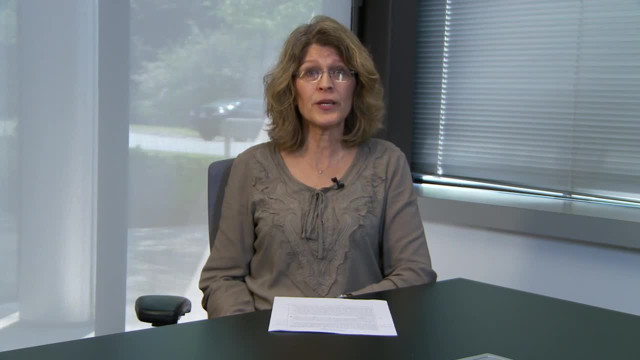 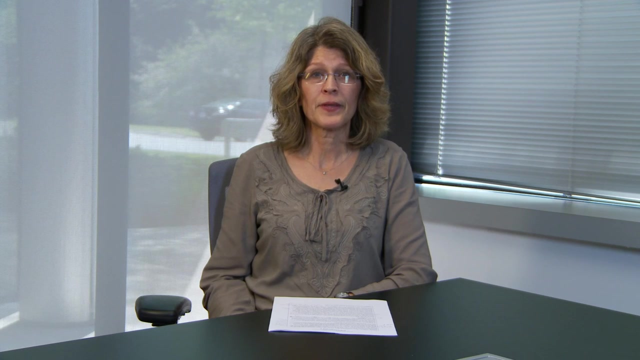 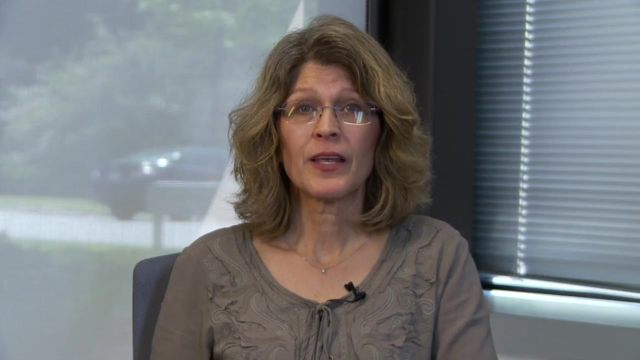 Thank you. the glitter, because I find that really messy and I never use the ventilation hood or the centrifuge tube, but I still get across the same process. you want to use it with whatever is available in your classroom. ultimately, the only components that are critical to the glue making process are the milk, the vinegar,